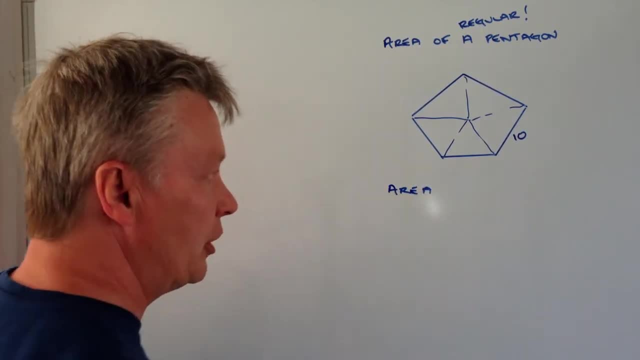 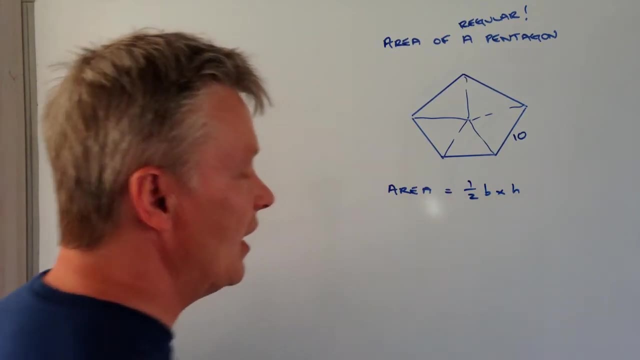 Well, area of a triangle. there's a couple of formulas you can use, but the most popular one at the moment for this is going to be a half base times height. So if we look at this individual triangle and we take this out, what we've got is something with a base. 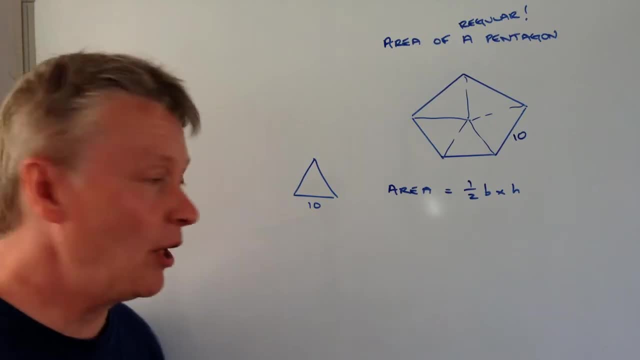 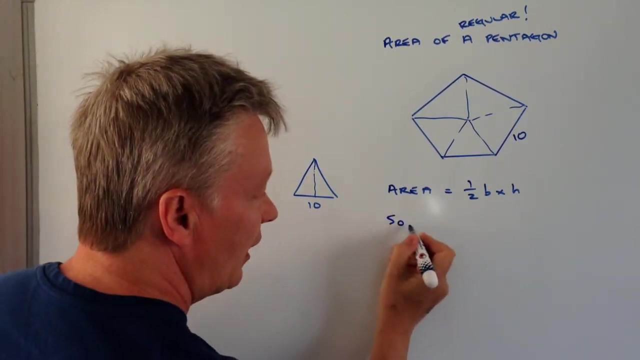 of 10, which is this one here. perfectly fine, but unfortunately we don't actually have that height and we need to figure that out. Well, we're going to use the other area of this, which is going to be SOHCAHTOA, or trigonometry, to be able to work out that height, because 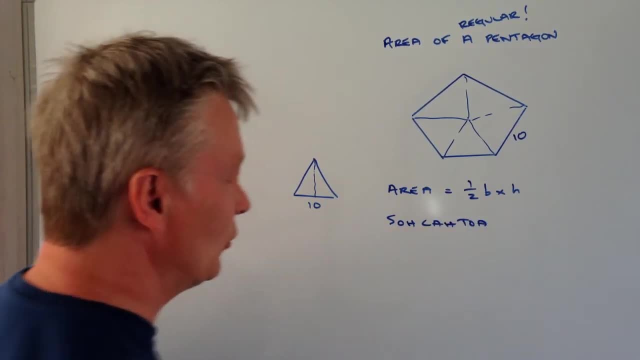 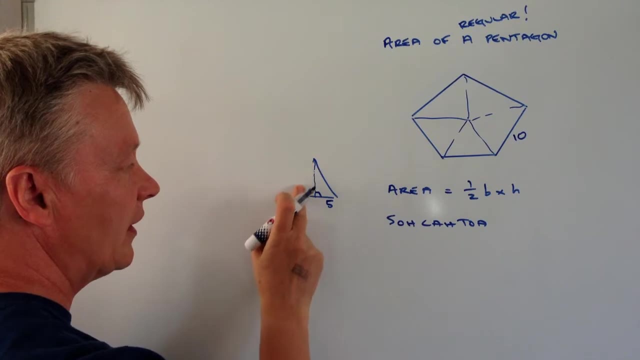 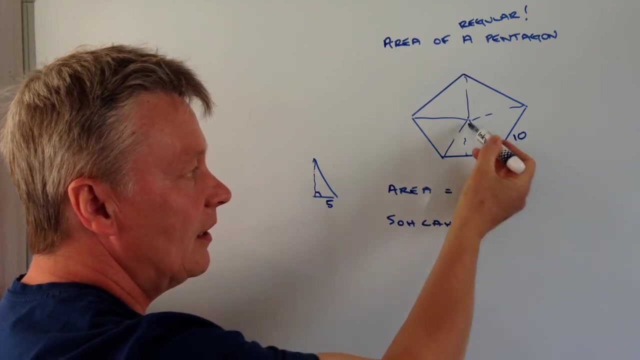 we can create a right angle triangle from this just by saying, well, the base is now 5 and that's a right angle, and I can get rid of that. And what I do know, then, is that if I take this right angle triangle here, just half of one of these triangles, then I can. 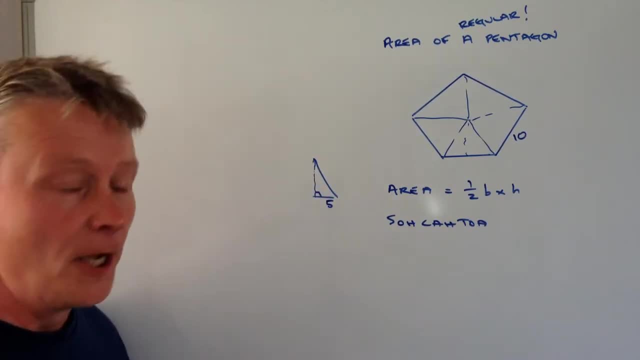 use SOHCAHTOA to work out the vertical, The vertical height, Because I can also find out the angle at the top. here The angle at the top is going to be 360 degrees divided by 5, because there's 5 triangles. So in other 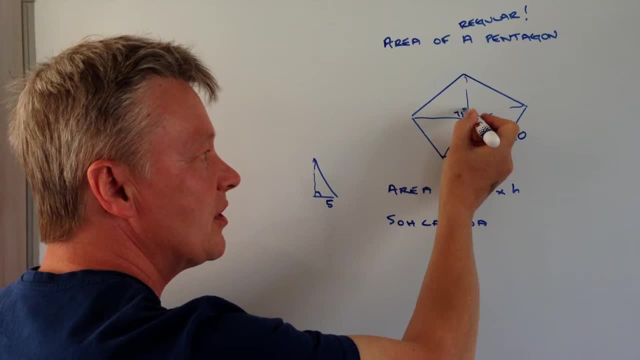 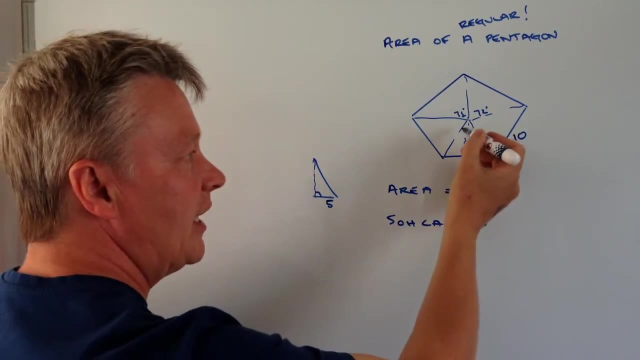 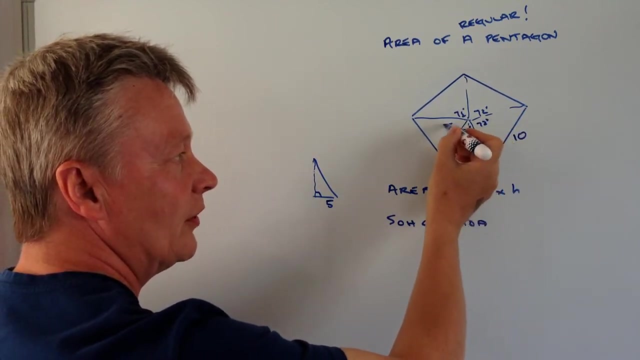 words, each one of these angles at the top is 72 degrees, And if you pop that into a calculator, you'll be able to just divide 360 by 5, and each one is 72 degrees. So therefore, if we've got this right angle triangle that we've created here, it means 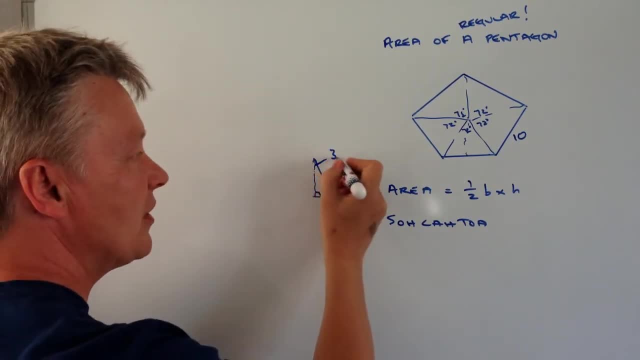 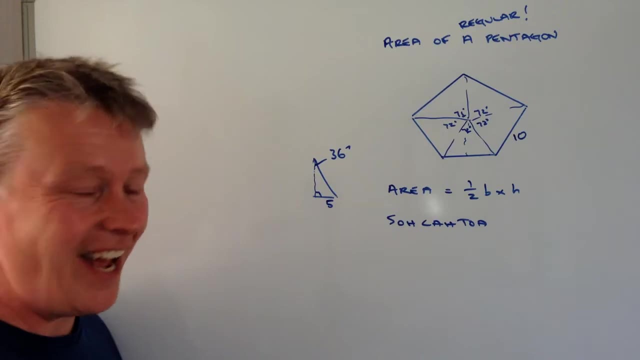 this bit is going to be half of that, which is 36 degrees. Okay, so I'm now in a position where I can use SOHCAHTOA, and the relationship I'm going to use is tan, because this is the opposite and this is the adjacent, and it's actually. 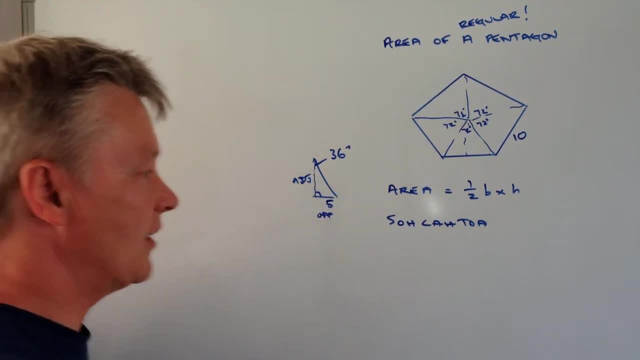 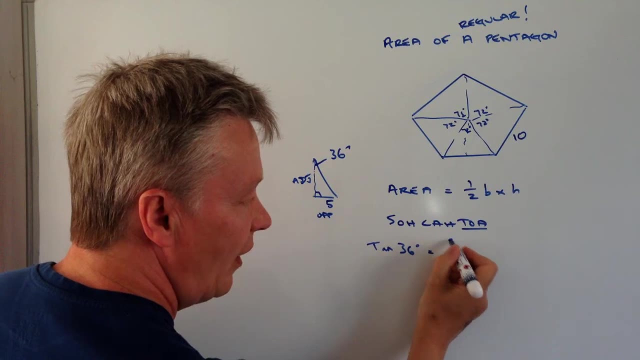 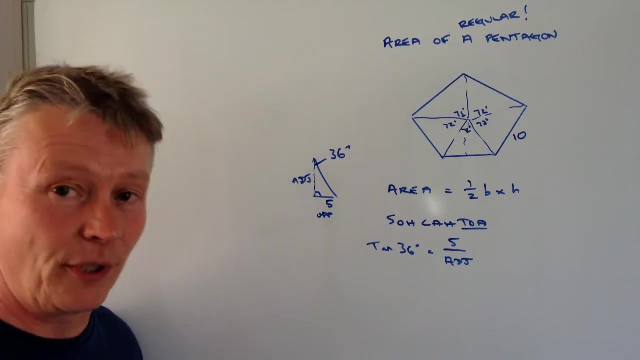 the adjacent that I'm looking to find out. Okay, so let's look at that: 36 degrees equals the opposite, which is 5, divided by the adjacent, which is the bit that I'm looking to find out, And I can now use a little bit of algebra to be able to move these around, So I can. 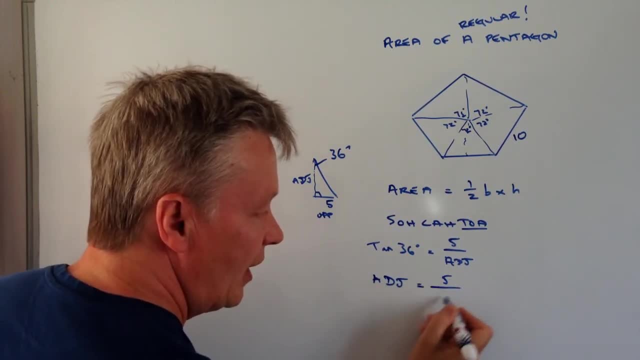 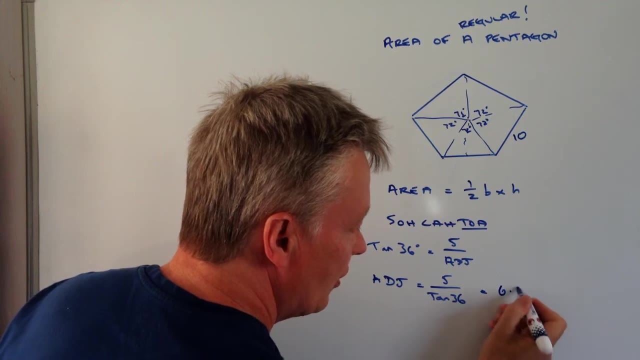 pop that into my calculator as adjacent equals 5 divided by tan of 36.. And if you do that, you're going to get 6.882.. Okay, That tells me, then, that the actual height of one of these triangles is going to be 6.882.. 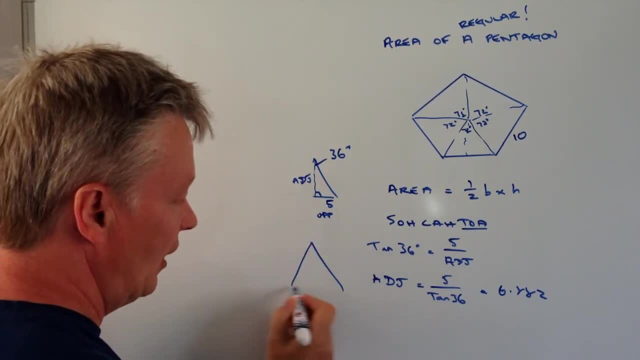 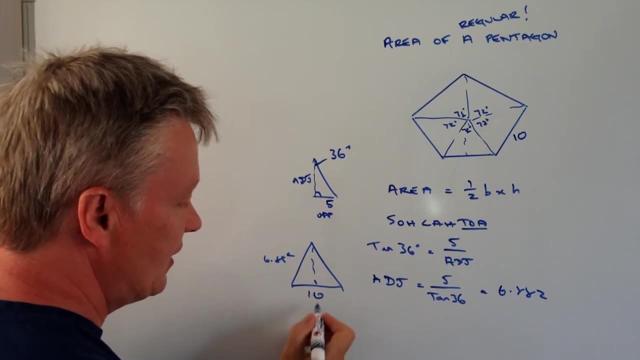 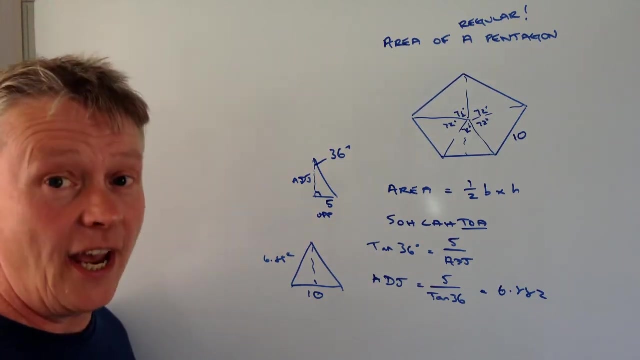 So now, if I redraw this triangle, the height is going to be 6.882 and the base is going to be 10.. Okay, So now I'm in a position where I can go back to using this formula, which is: area equals. 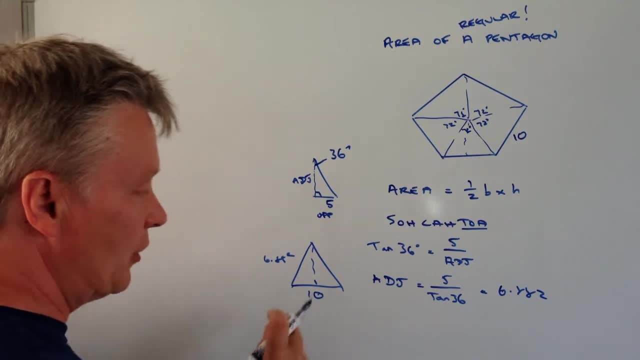 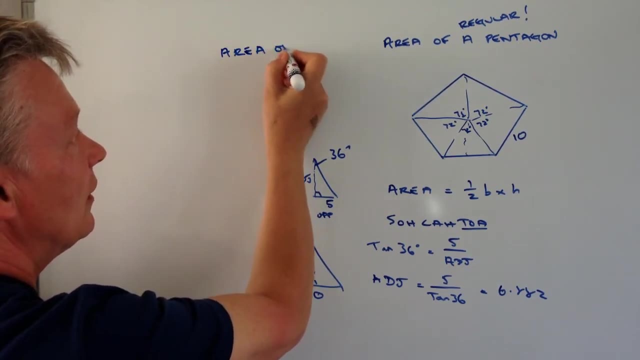 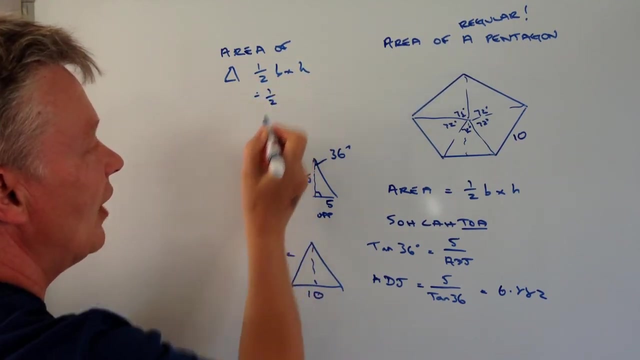 a half base times height. Well, if I use my calculator then to figure that out, I could just write it up here. So the area of a triangle, Okay, Is going to be a half base times height. Well, that's going to be a half, and the base 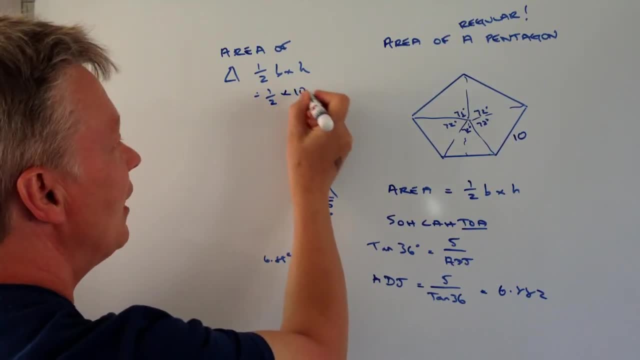 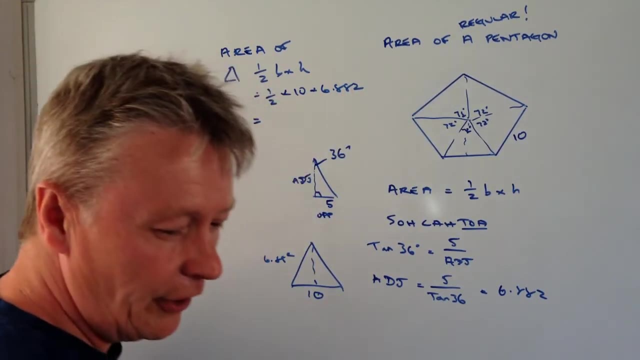 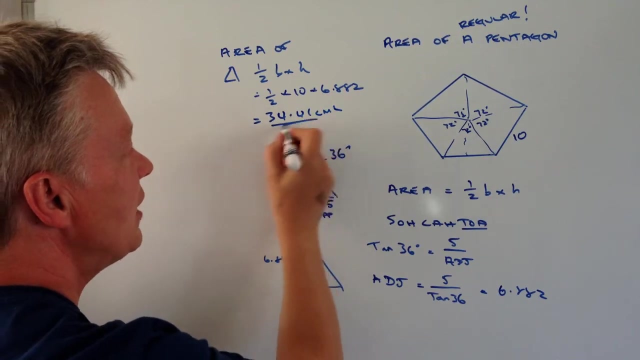 is going to be 10 times 10 and the height is going to be 6.882.. Now, if I put that in my calculator, I get a total area of 34.41 centimetres squared. So in other words, each one of these triangles is 34.41.. 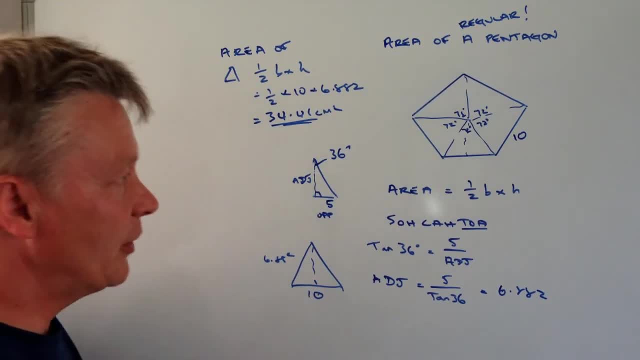 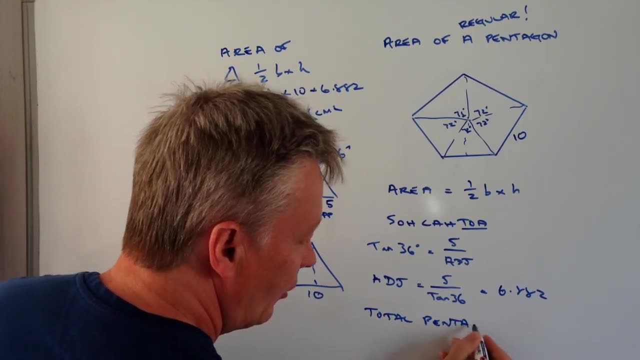 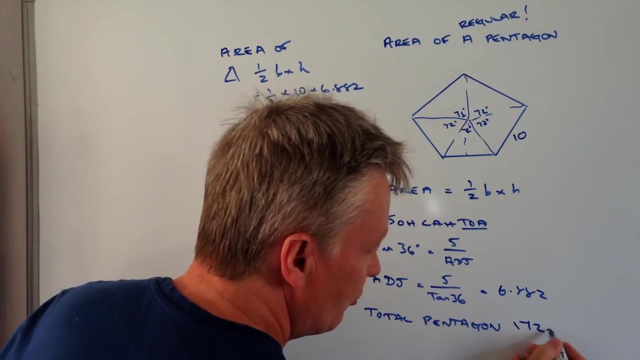 If I then multiply that by 34.41.. If I then multiply that by 5, I'll get a total area of the Pentagon. Total Pentagon area, okay, is going to be 34.41 multiplied by 5, which is 172.05 centimetres. 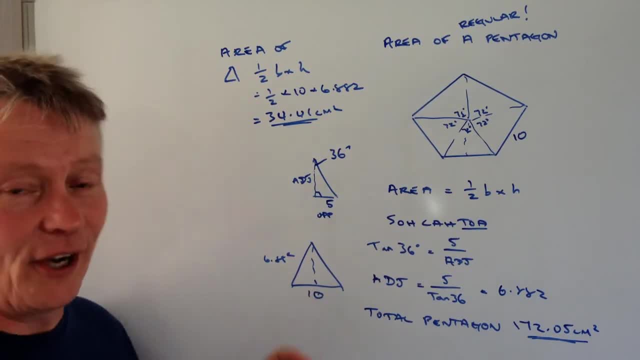 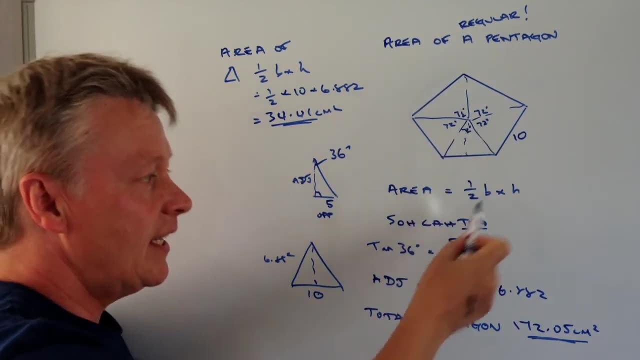 squared, Okay, So it's a little bit of a jumble on the board here, but hopefully you get the idea that what we're doing is breaking this regular Pentagon down into a triangle. Okay, We're using Sokotoa, So this is your first point. 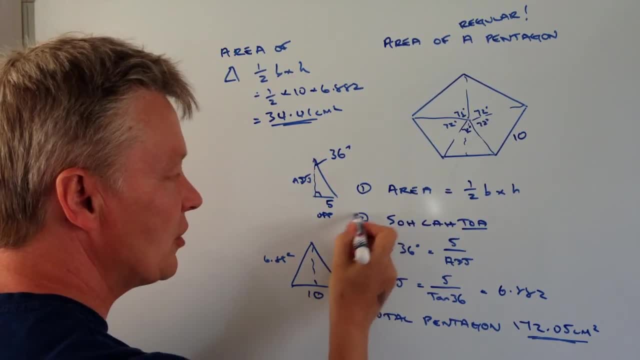 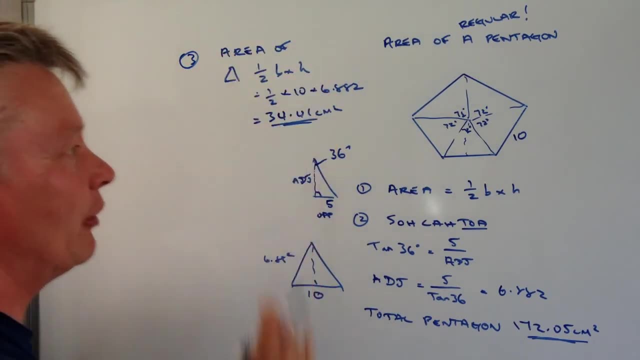 This is the information we need. The second point is we're going to use Sokotoa to actually work out the information that we need. The third thing is we'll work out the original area of one particular triangle And then the fourth thing is that we multiply it through and get the total area of the Pentagon. 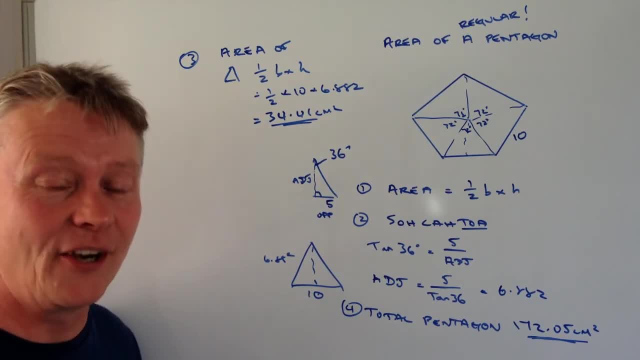 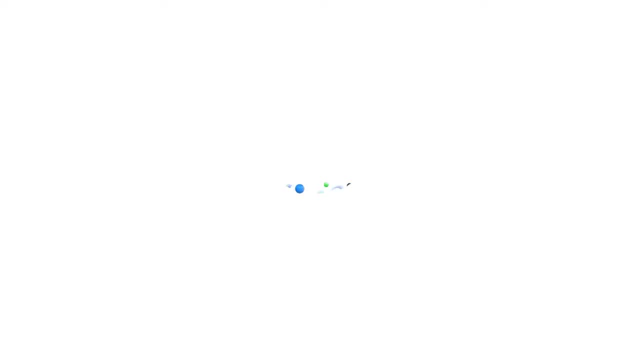 I hope that's been okay for you. Please do add a comment below in the comments. I'll always come back to you. Look forward to seeing you inside the next video. Bye everyone. Thanks for listening. I'll see you next time. Bye-bye, Bye-bye.